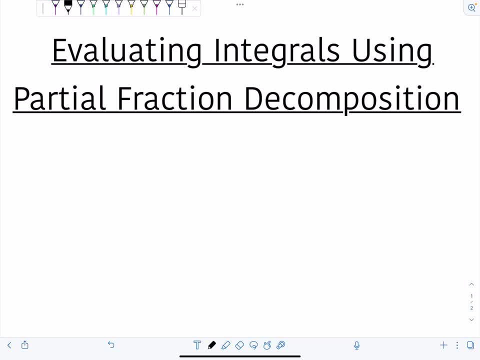 and be able to work with. So the purpose of this video is just to work through some more examples and work through some more spicy integrals, as I like to call them, the fun ones. So let's get started. First example: here we have indefinite integral, 3x squared minus 11x plus 4 over. 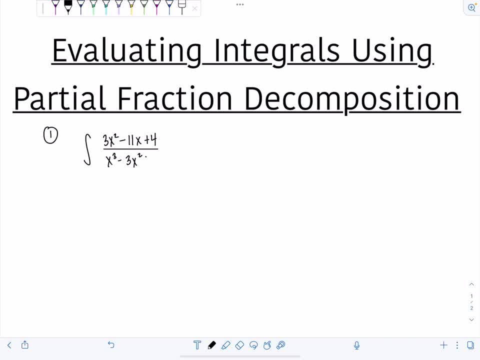 x cubed, Minus 3x squared, plus 2x dx. All right, so first things first. I notice I have a rational function. Degree of the denominator is higher than the degree of the numerator, So I can proceed with the partial fraction decomposition. In order to do so, we have to factor the denominator first. 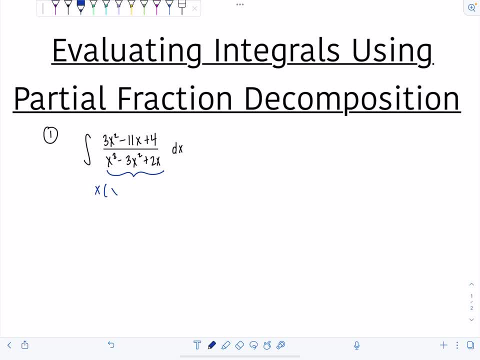 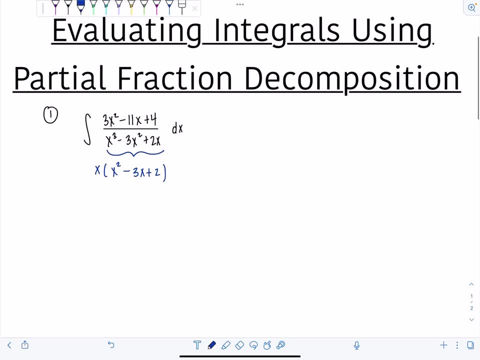 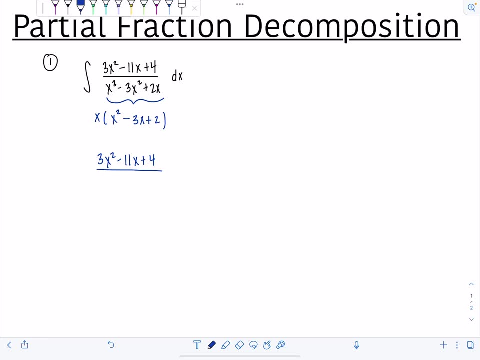 completely. So notice, I can take an x out from all the terms and we'd have a partial fraction of x squared minus 3x plus 2 left over, and that factors further. So now I'm going to write everything out: We have 3x squared minus 11x plus 4 over x times, and then I need to factor. 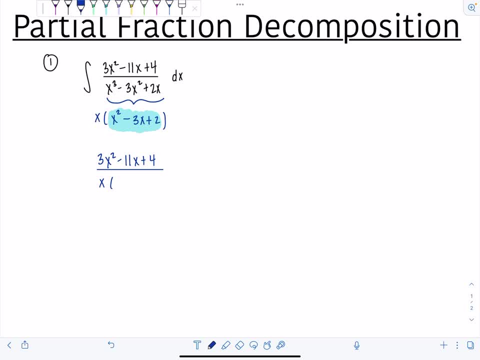 this trinomial here, which is going to factor into x minus 2 times x minus 1.. All right now, looking at each of the factors in the denominator, all linear meaning, x is raised to the first power and none of them are repeated. So this is one of the 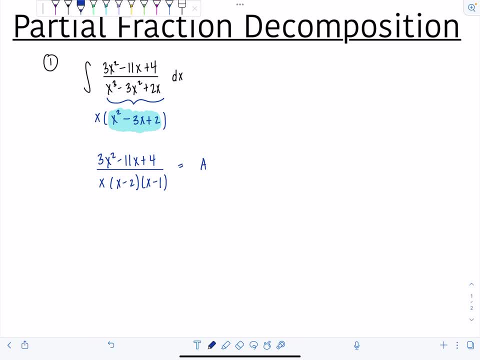 most straightforward cases. I'm just going to have constants in each of the numerators here for my decomposition. So a over x plus b over x minus, 2 plus c over x minus 1.. Nice, Now, in the next step, you want to clear out all your denominators. 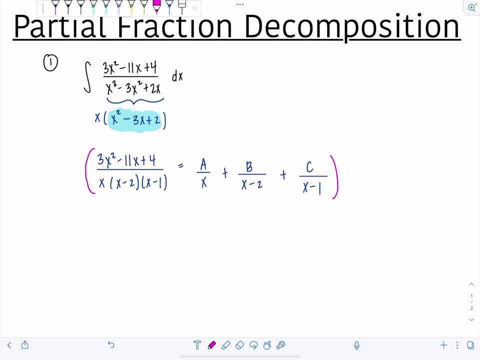 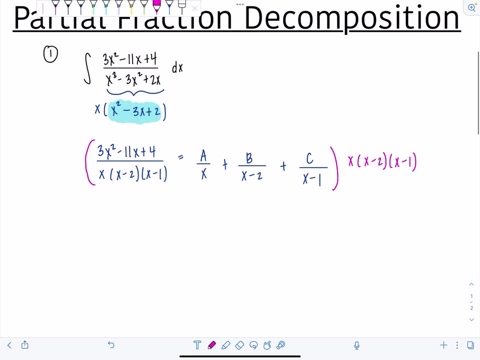 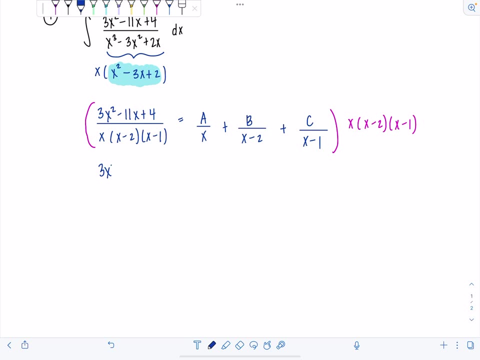 We're going to multiply by LCD. In this case that's x times x minus 2 times x minus 1.. And everything in this equation gets multiplied by that. So on the left hand side now we're just going to be left with 3x squared minus 11x plus 4.. 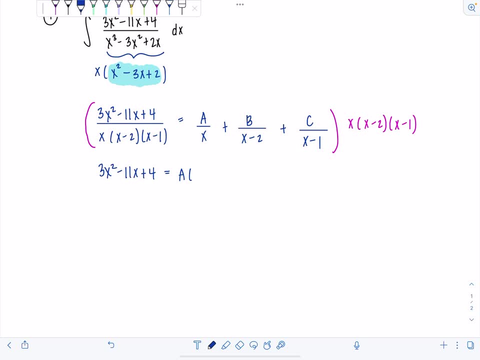 And then on the right hand side we'll have a times x minus 2, times x minus 1.. Plus b times x. Notice the x minus 2 will cancel. So I just have x minus 1 left, plus c times x, times x minus 2.. 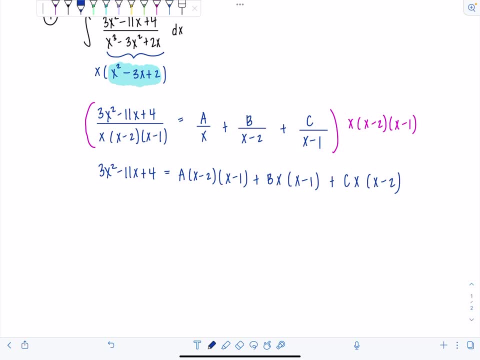 All right, This is a good place to pause. You have the option of multiplying everything out, but I think it's easier if we use a different method to try to solve for a, b and c by substituting different values of x. that would make each of the factors zero. So first one we can try is letting 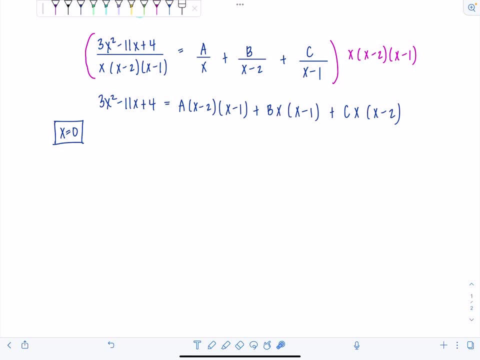 x equal zero. Why did I pick that? Well, if I let x equal zero, notice here- this entire term and this entire term will go to zero. So you're going to substitute in values for x. that would make each of these factors of the original denominators zero. All right, so if x is zero on the left hand, 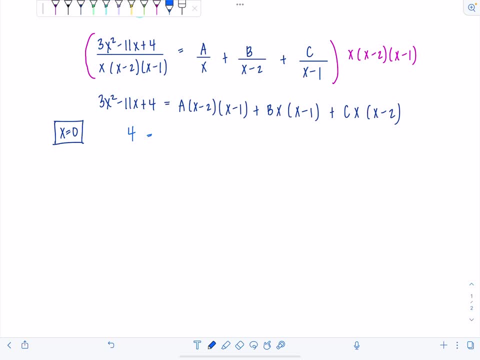 side, we're just going to be left with a four, and this is going to equal a times zero minus two, that's negative two. zero minus one, that's negative one plus this whole term is just going to be zero plus this is zero. All right, so then, if I simplify further, we have: four is equal to two a. 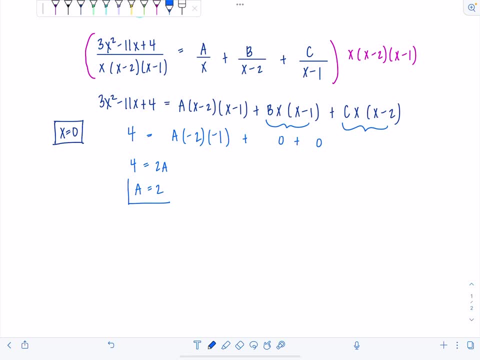 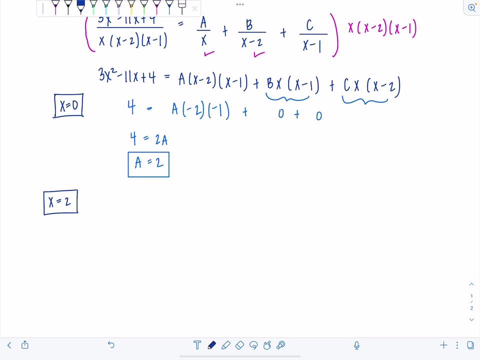 so a is going to be equal to two. So save that, and then we're going to repeat the process. So now we let x equal zero, then we can let x equal two. So let's go ahead and substitute in two for x. Where do you substitute that in? 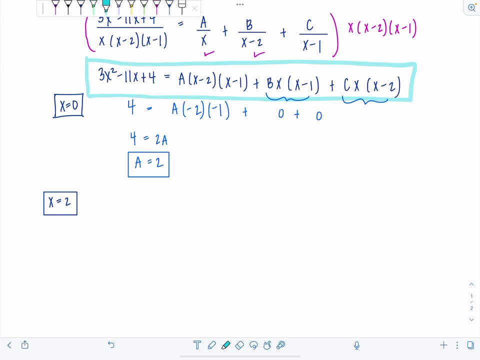 After you've cleared out the denominators from the equation right here. Okay, so I'm going to plug in two for x now. So we have three times two squared, that's three times four. so twelve Minus eleven times two, that's twenty two plus four. What's that going to equal? Well notice, if I plug in two for x, this factor here is going to be zero. So this whole term is gone. Bye, bye. 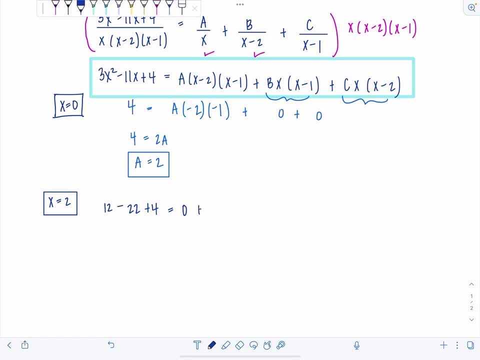 So we've got a zero plus b times two. right, we're plugging in two for x, and then two minus one, that's two, that's one plus, And this last whole term is going to go to zero because we're plugging in two for x again, remember, 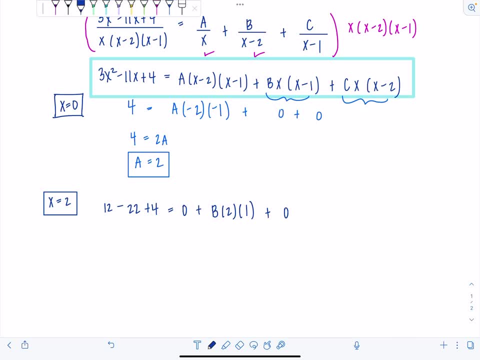 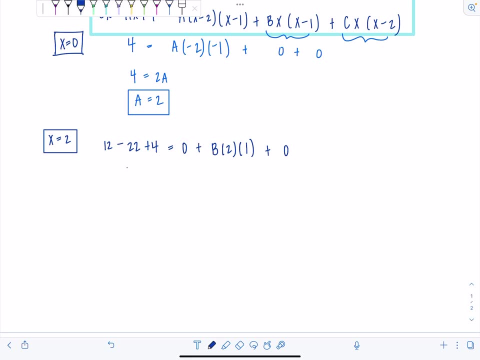 Zero. All right, Love it. On the left hand side we've got twelve minus twenty two, that's negative. ten plus four, that's negative. six equals two b. so b is equal to negative three. Okay, almost there, Last one. What do we need to let x equal, Can you see? 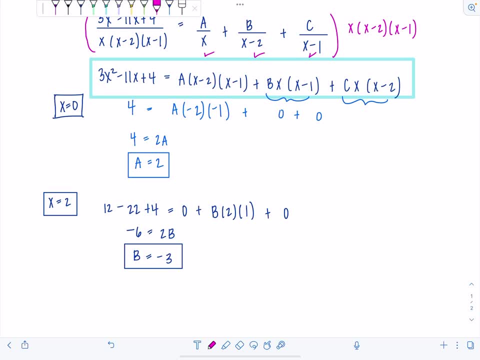 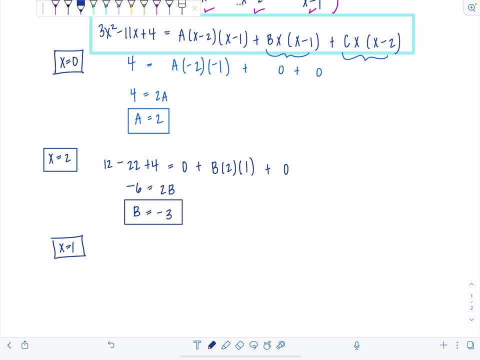 Why, yes, We need to let x equal one. Bravo, So we're going to let x equal one, And then now substitute that back into the blue equation that I boxed after we cleared the denominators. So if x is one, we'll have three times one squared. so that's three minus eleven times one, that's eleven plus four. 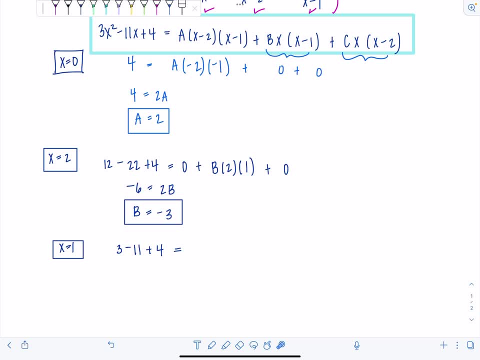 Equals. Now, remember: x is one, so this factor is going to be zero, wiping out this whole term. Bye, bye. Plus again, x is one, so this second term is also going to be gone. Plus we have c times one times one minus two, that's negative one. 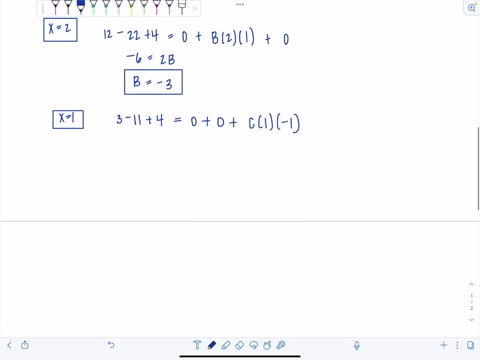 All right. Now let's see: Three minus eleven: That's negative. eight plus four: That's negative. four equals zero plus zero. That's going to be negative c left over on the right hand side, which tells us c is equal to positive four. 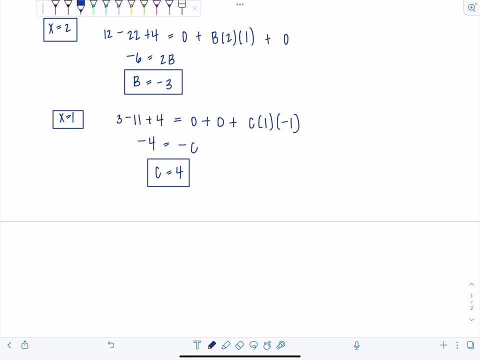 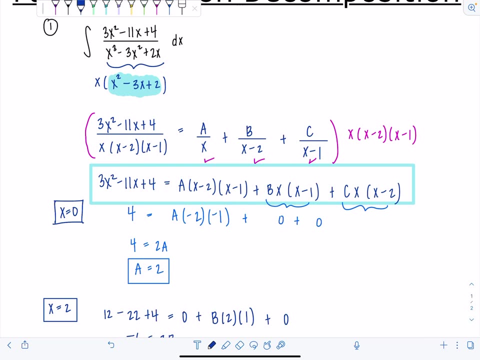 Okay, great, That one wasn't too bad. So now we're going to go back to the original integral And what I'm going to do is replace the constants a, b and c with the values that we found. Remember, a, we found, was two, b, we found, was negative, three and c was four. 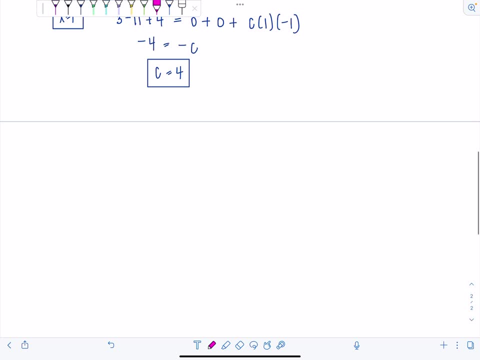 So I'm going to rewrite the original indefinite integral using my partial fraction decomposition. So we have now the integral of two over x, since a was two, b was negative three, So that's minus three over x minus two Plus four over x minus one dx. 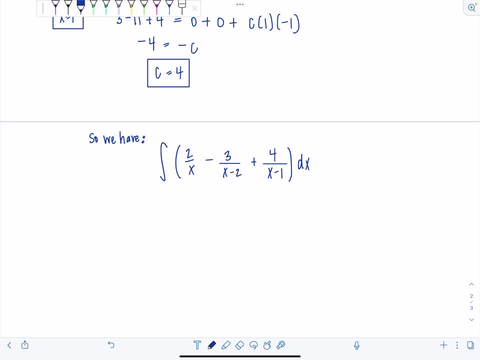 All right, Now can we anti-differentiate each of the terms that we see here For sure, I mean, they're all just basically going to be ln- absolute value of whatever's in the denominator, And then just throw these constants out front. 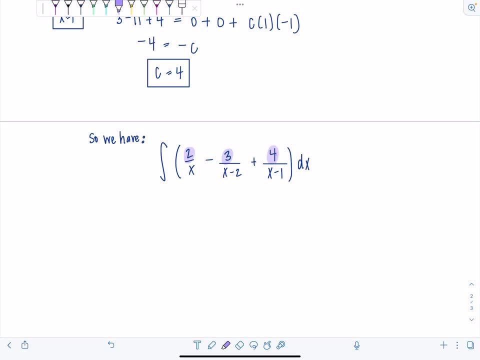 Right, No u sub or fancy maneuvers necessary, So we can just jump straight to the final answer. Okay So anti-derivative of two over x would be two natural log absolute value of x, And then minus three natural log absolute value of x minus two. 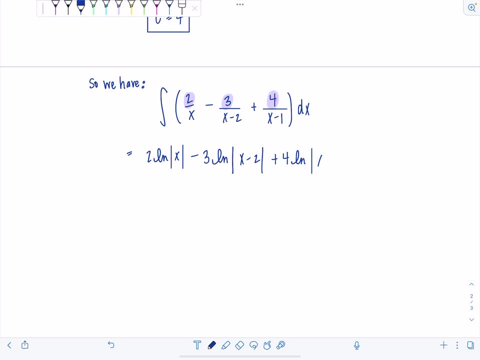 Plus four. natural log absolute value x minus one, And don't forget to put plus c. All right, How was that one? Did you love it? It was pretty straightforward. It's a basic example. I just wanted to get us all warmed up. 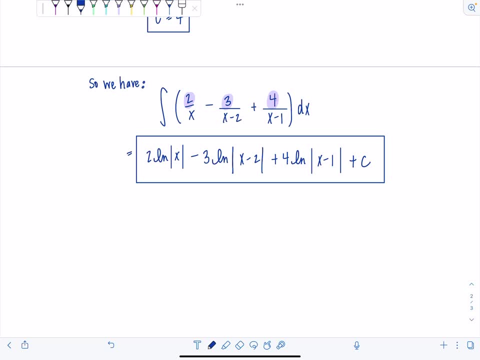 The next three, the spice level will increase. Okay, So this was just like a crunchy pepper. I've got a jalapeno coming up And then we're going to bust into a serrano at the end. Okay, Yes, All right. 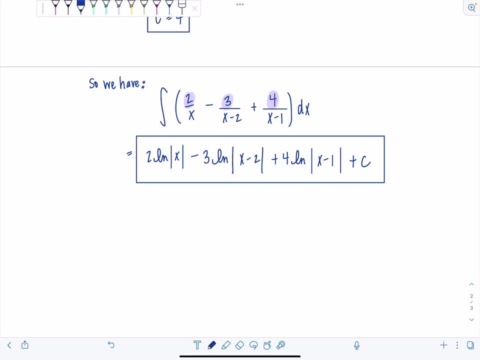 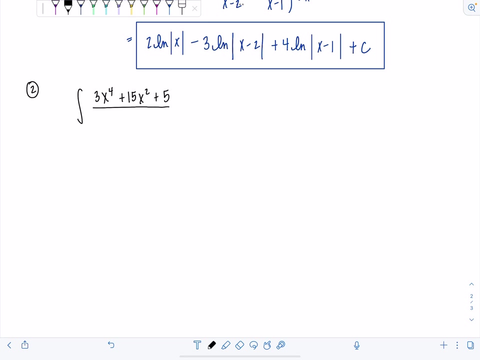 So next one I want to look at here: Example two. These are all going to be indefinite integrals, just so we can focus on the technique, But you can also do definite integrals with these. We've got three x to the fourth plus 15, x squared, plus five over x cubed, plus five x dx. 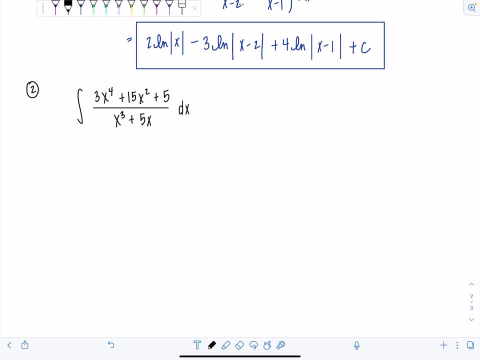 All right, I have a rational function, But do you see how the degree of the numerator is degree four, whereas the degree of the denominator is only degree three? That means it is not time to do partial fraction decomposition yet. Oh, no, no, no. 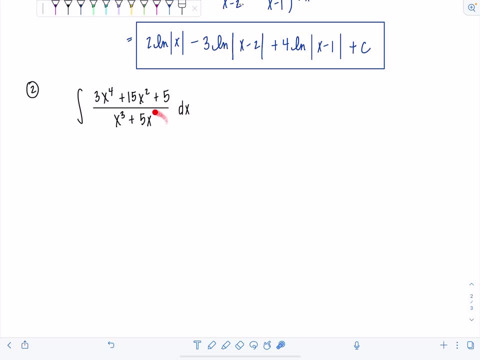 The degree of the denominator needs to be higher than the degree of the numerator when you apply a partial fraction decomposition. So if it's not, you must long divide first. All right, first. did you forget how to long divide polynomials? have no fear, I'll link a. 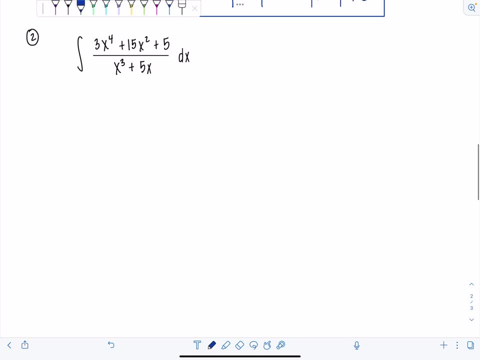 little video here that'll get you through a little refresher. okay, it's not too long. I'm just gonna assume you remember, okay? so here we've got X cubed. I need a 0x squared as a placeholder, and then we have 5x and then we have no. 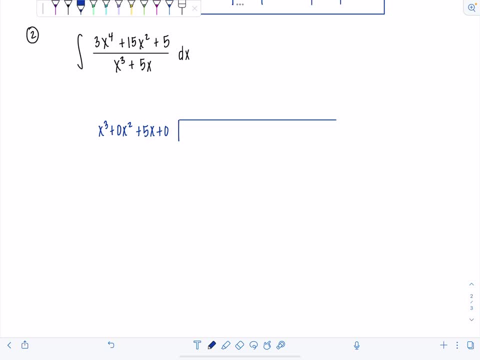 constant and this is gonna get divided into 3x to the 4th plus. I need a placeholder for that: X cubed plus 15x squared plus 0x plus 5. all right, remember, when you're doing polynomial long division, you only look at the. 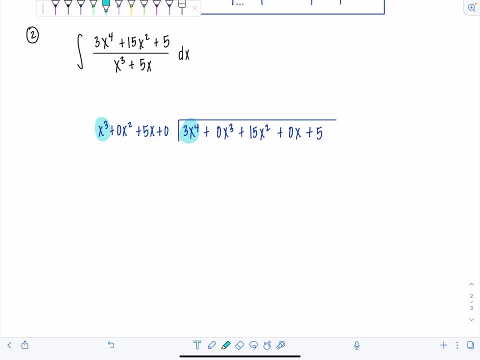 leading terms. so just think to yourself: why do I have to multiply X, cubed by, to make it 3x to the 4th? that's right, just a 3x. and then that 3x gets multiplied by everybody in the divisor. everyone's sitting outside, so we have 3x to the 4th plus this would be 0. 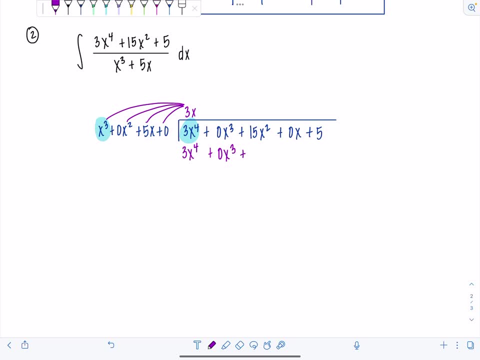 X cubed plus 5x times 3x, that's 15x squared plus 0x. nice, then we subtract the bottom of the denominator from that. so 5x multiplied by 15x, squared 3x times 3x, that's 15x squared plus 0x. nice, then we subtract the bottom of. 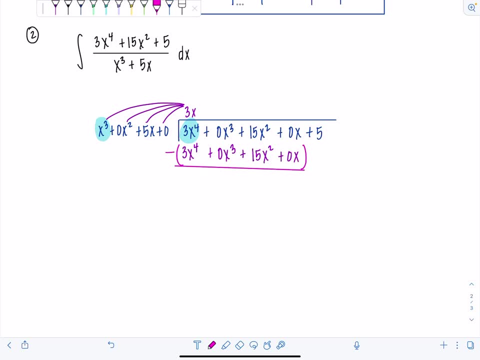 row from the top row. The furthest left terms should cancel out. And then the second term is also canceled. This cancels, This cancels. So we're pretty much done. Bring down the 5.. And this is our remainder. How do I know it's a remainder and I can't keep dividing. Well, 5,. 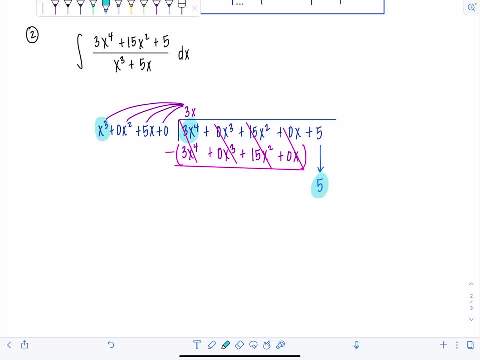 that's just a constant. It's degree 0, right, There's no variables attached to it, And our divisor sitting out here is degree 3.. If the divisor is a higher degree than whatever you're left with, you are done. That's your remainder, Okay. So how would you write out the result? 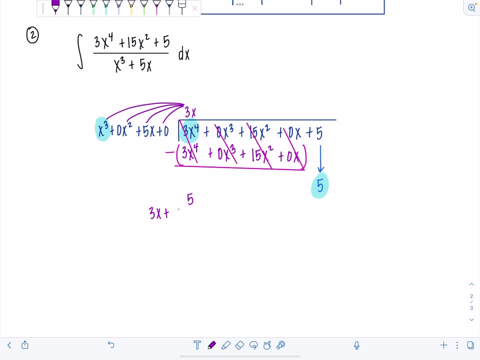 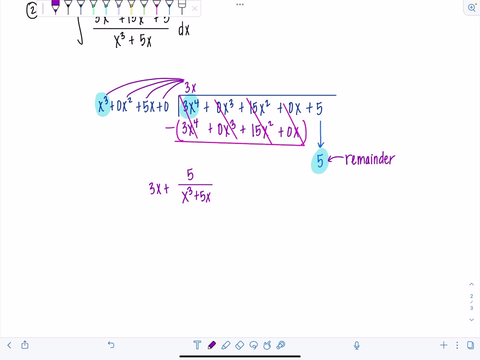 It's 3x plus 5 over. what were we dividing by x cubed plus 5x? You don't have to put all the placeholders in for your final answer. Okay, So this is your little remainder. It looks so harmless. Okay Now, if we're going to integrate what we found here as a result of 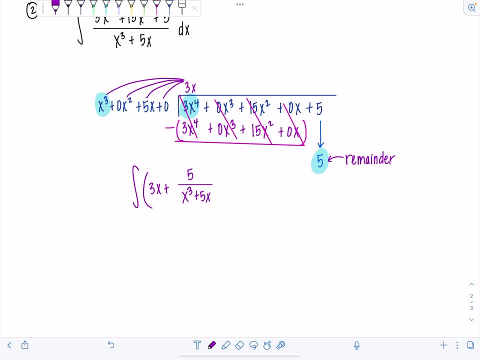 doing the long division, we still need to apply partial fraction decomposition to the remainder portion. right, You know how to integrate 3x, That's no problem, We got that. Should I put a little happy face? Yay, But 5 over x cubed plus 5x. Ooh, yeah, We need to do partial fractions. 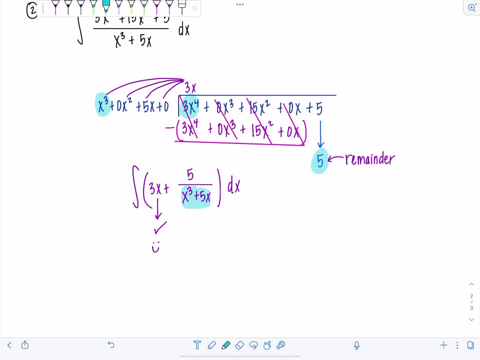 in the numerator right. Can't u sub? sadly right, If I let that be u I would need. too bad. there's no 5x squared in the numerator right. Oh man, It's fine. That's why we got partial fraction. 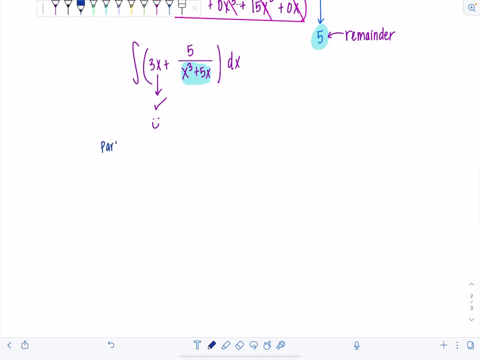 decomp to save the day. So here we go. It's partial fraction time And remember you need to factor that denominator completely. So 5 over x cubed plus 5x, How would you factor that? 5 over x cubed plus 5x, How would you factor that? 5 over x cubed plus 5x, How would you factor? 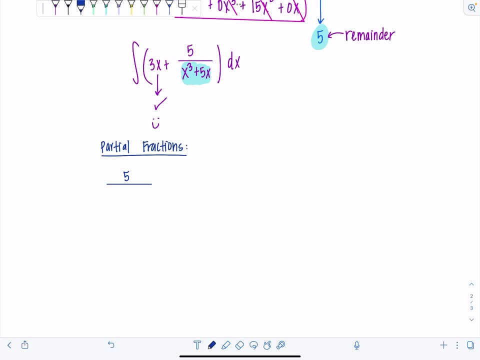 that, Yep, Just take an x out, So you've got x times x squared plus 5.. And so our setup for this case would be a over x plus notice: x squared plus 5, that's an irreducible quadratic. So the 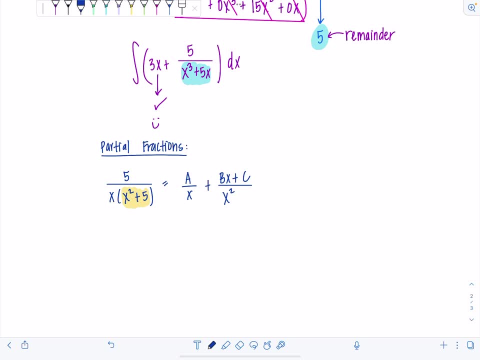 form bx plus c. Again, if you forgot about this, that's in that video that I linked earlier, just explaining how to do partial fraction decomposition. Okay, From here the next step is the same as in the first example. You're going to multiply everything by the LCD. 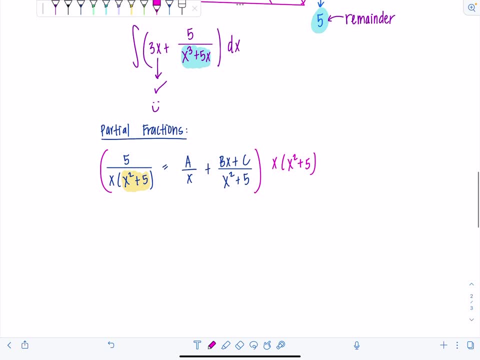 which is x times x squared plus 5.. You want to be fraction free, So on the left-hand side we're going to have just 5 left over, equals a times x squared plus 5.. So this is going to be a over x plus bx plus c times x. Good, Good. Now, if you'll notice here, 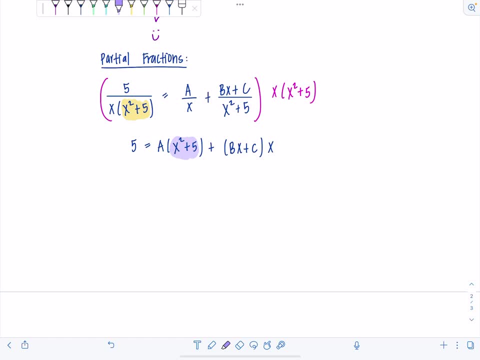 since we have an irreducible quadratic, there's nothing that we can plug in for x that would make that first factor equal zero. right, We'd have to use imaginary numbers and we're not working with those right now. So another technique to try to solve for the constants is to multiply everything. 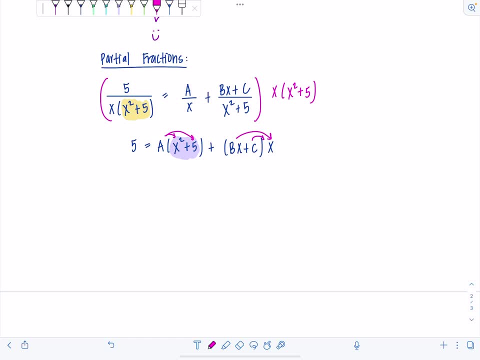 out. Okay, Do, do, do, do, do So let's do it. So we've got 5 equals ax squared plus 5a, plus bx squared plus cx. And what you do to proceed from here is you collect the coefficients for like terms. 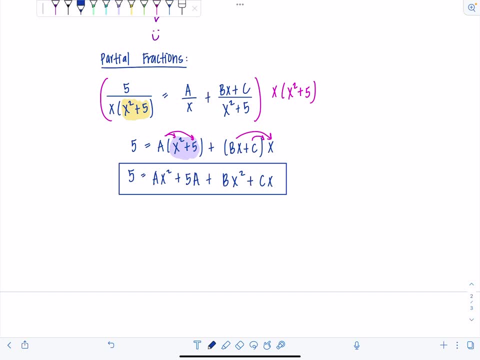 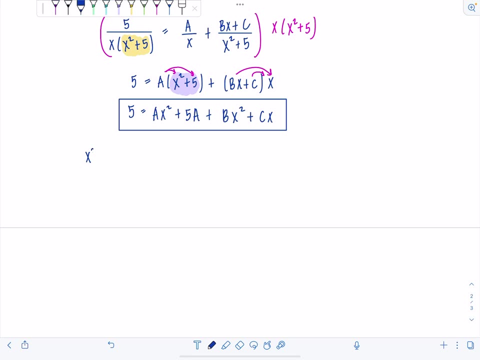 on both sides of the equation and set them equal to each other so you can solve. What am I talking about? I'll show you, Don't worry. So find all the terms on the left-hand side that are coefficients of x squared. So you might be thinking I don't know what you're. 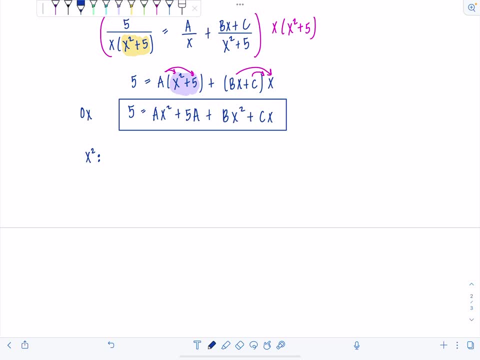 talking about. There's no x squareds on the left-hand side. You're correct, There's a zero x squared on the left-hand side, So zero must equal. where are the x squareds on the right-hand side? Well, I have an ax squared and a bx squared, So zero must equal a plus b, right? 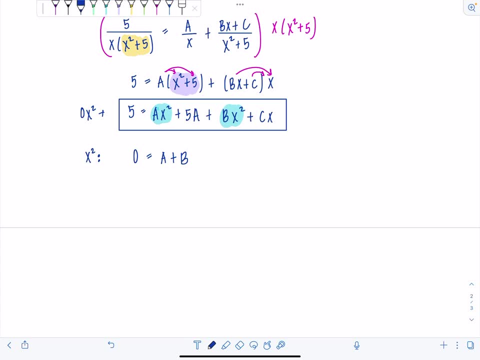 The coefficients of the like terms must be equal on both sides of the equation. What about x? Do you see any x's on the left-hand side? Nope, me neither. So you've basically got a zero x hiding there. What terms involve x to the first on the right-hand side? 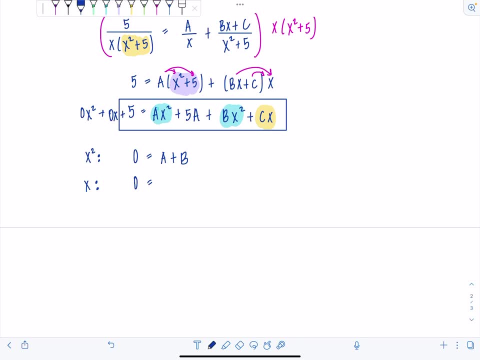 Only this last one, cx. So that means c must be zero. And then, last case, would be your constants. So on the left-hand side, I do have a constant, I do have a constant. I do have a constant, This time five. And what's my constant term on the right-hand side? 5a, That's the term that 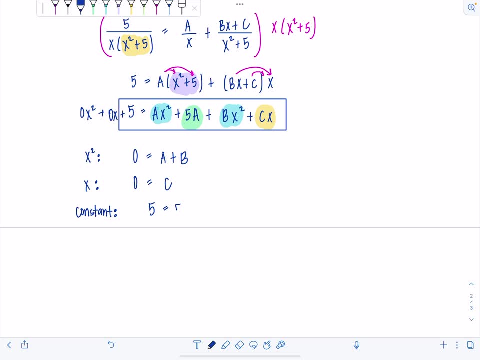 doesn't have any x's attached to it, right? So it's a constant. Well, that tells me, a is equal to one And remember, I already know, c is zero. And if a is one, since a plus b is zero, then b. 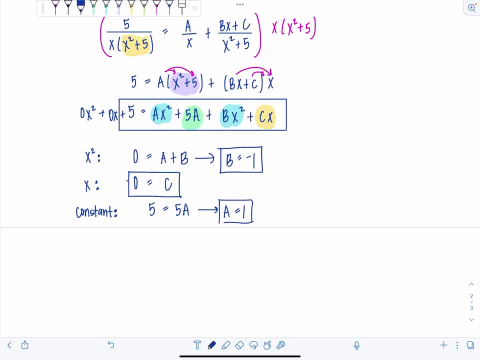 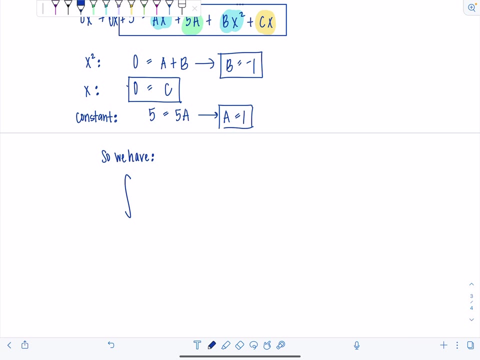 must be negative one. And now, basically, we're done with the partial fraction decomposition. So that's an alternate approach that you could use. Okay, so now let's put everything together. What do we have now? Do you remember from the long division? we have that 3x hanging out first. 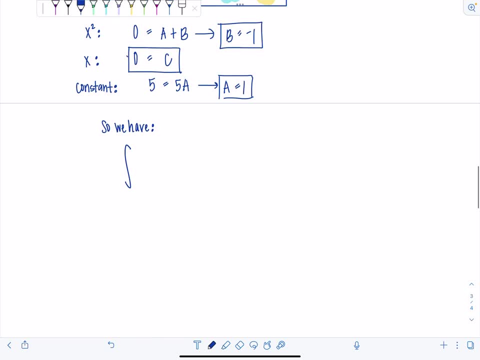 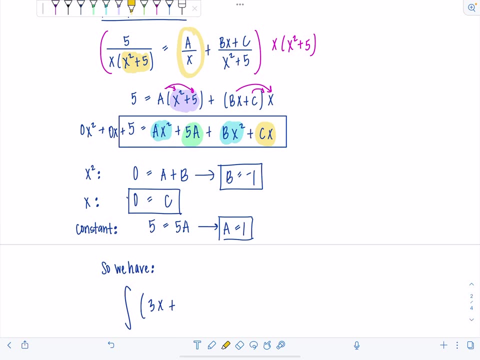 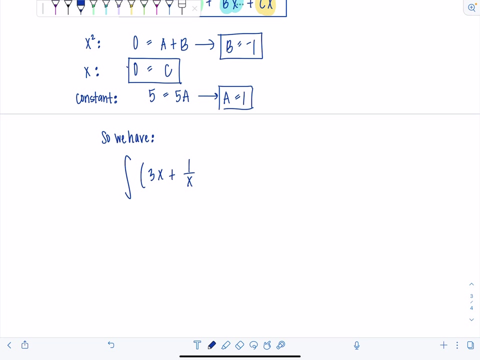 Don't forget about it: 3x. So we've got 3x, plus a was one. So this is going to give us one over x, And then b is negative one. So I'm going to put minus x over x, squared plus 5 dx. 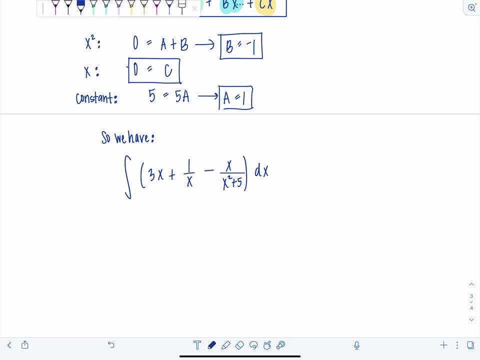 All right, now let's see how we would anti-differentiate each of these. 3x- no problem. 1 over x- no problem. x over x squared plus 5, that's no problem, but we're going to have to. 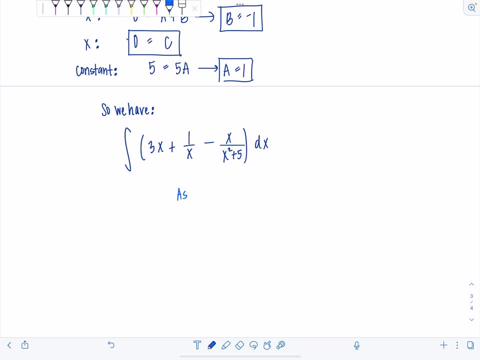 use substitution. So let's do a little aside. If you have integral of x over x squared plus 5 dx, I know to use u substitution because the denominator is degree 2. And you see how the numerator is one degree lower. That's the most. 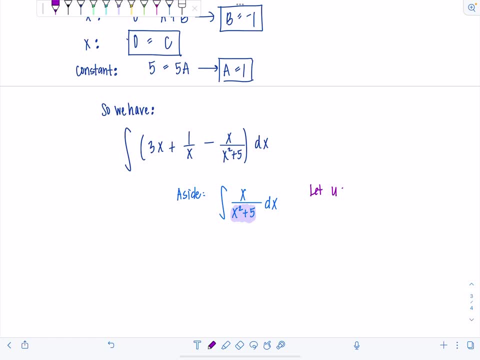 perfect time to use u substitution, Because if I let u equal x squared plus 5, then what's du going to be? Mm-hmm, It's 2x dx, Which is fabulous because we've got that xdx right there. So one half du is xdx. 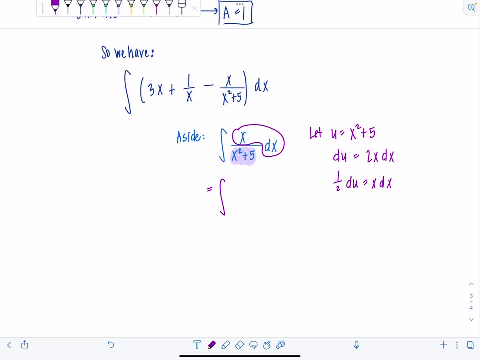 which means this is going to give us integral. I usually like putting the constants outside, So let's put that one half out there. du over u Mm-hmm, Mm-hmm. And then what would this be? This would be one half ln absolute value of u. 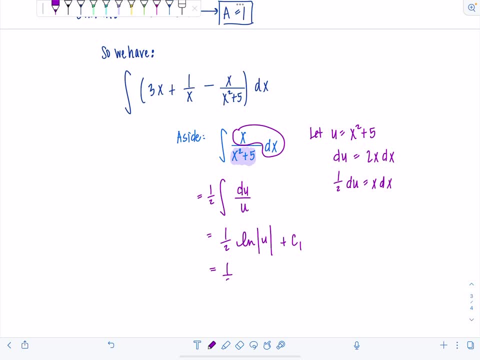 plus, I'll call it c1, which is one half ln absolute value x squared plus 5 plus c1.. Okay, Why am I calling it c1?? Because this is not my final answer. I want to save just writing plain old c for my last answer that I'm going to report, Which means now: 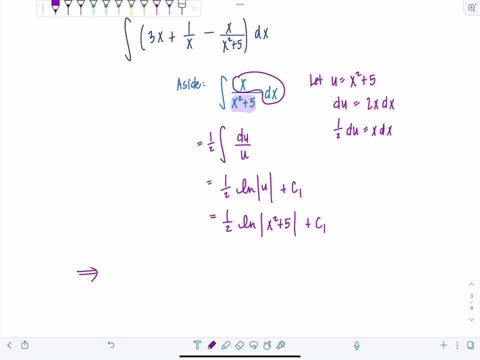 we have antiderivative of 3x Mm-hmm, 3 halves x squared plus what's the antiderivative of 1 over x ln? absolute value of x. Then we have minus, okay, all of this stuff that we had here, Minus one half ln, You know. 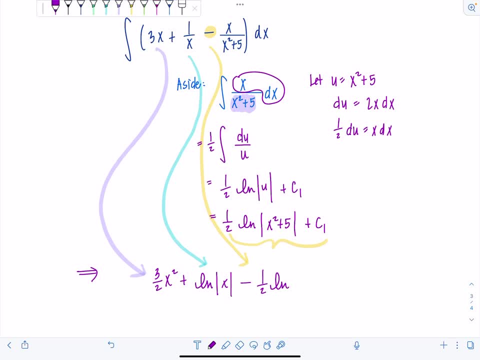 I don't need absolute value around x squared plus 5, because there's no way that's going to be negative, right? If you square something, it's not negative, And if you add 5, then we're good to go. So I can switch those to parentheses If you don't, it's not wrong, It's just not as clean. 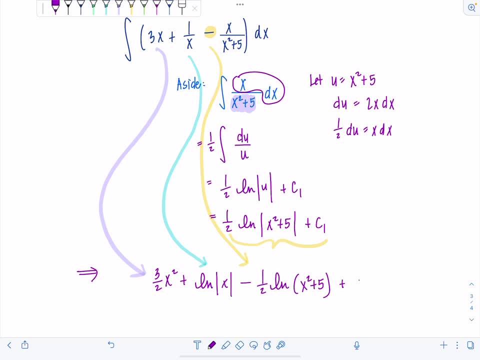 as can be. And then I'm going to put plus c. Okay, How was that? Now, when you get more practice with integrating, you might be able to identify that. oh, this is going to involve a? u sub. I'm just going to have a one half. I'm going to have ln- absolute value of the denominator, And 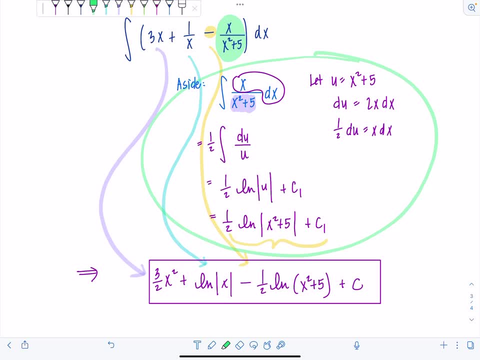 maybe you won't even need to write all this out aside, You can just do it in your head. I'm not even joking. Once you've done enough integrals, that's going to start happening to you. So if you're in my class, I have no problem. if you're going to skip those steps, But just check with. 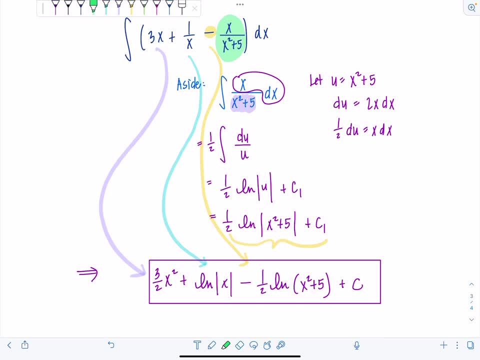 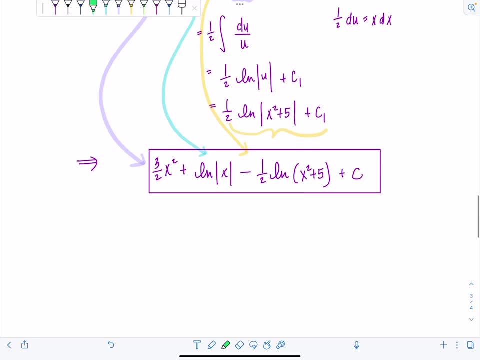 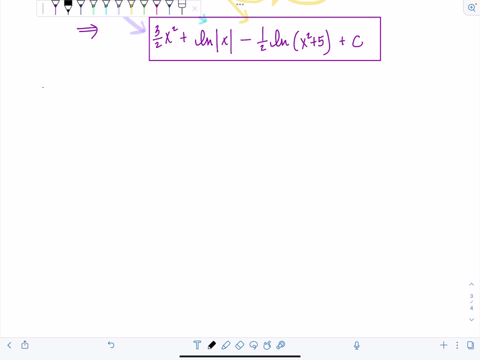 your professor before you take such liberties. okay, All right, nice, This was just, you know, moderately spicy Jalapeno. I've got a serrano for you, Oh yes, Example number three: Integral 3e to the 4t plus 12e to the 2t plus 4 over e to the 2t plus 4 dt. 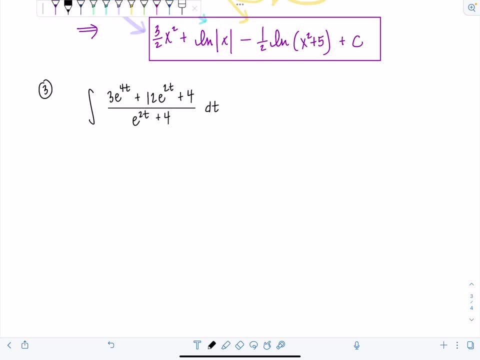 Okay, this one's going to take some manipulation. The numerator, I'm staring at it, staring at it and I notice these two terms. I can factor out a 3 and an e to the 2t from, But this poor little. 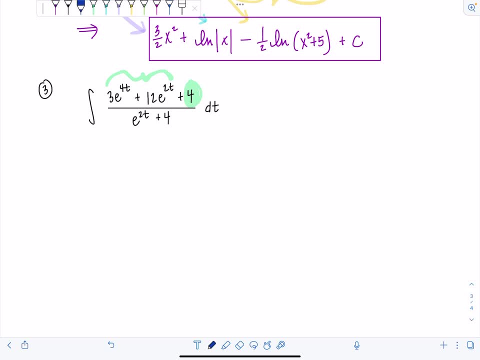 4, I can't do that with. So what I'm inclined to do now is split this integral into two. So I'm going to split it into 3e to the 4t plus 12e to the 2t over e to the 2t plus 4 dt. That's going to. 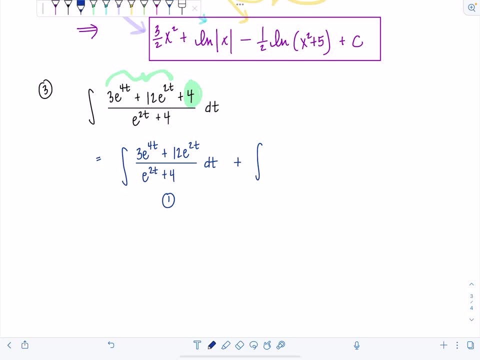 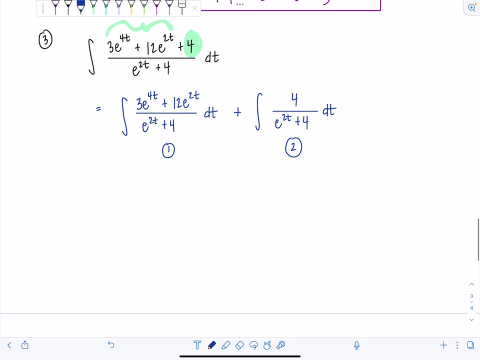 be integral one Plus integral two will be four over e to the 2t plus 4 dt. Okay, and we're going to tackle each of them separately. I know integral one looks more frightening, but it's actually way easier than the second one. So check this out. For integral one I mentioned initially, we can. 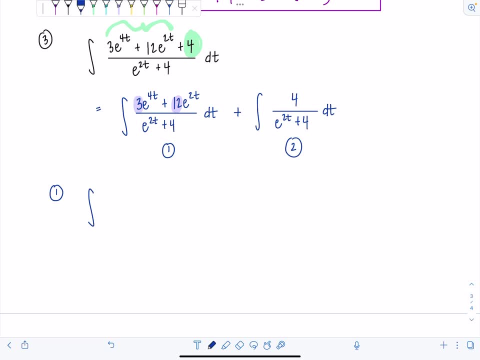 factor out a 3 from both those terms and an e to the 2t. So if I do that, if I take out 3e to the 2t, then what am I going to be left with in the numerator If you take out e to the 2t? 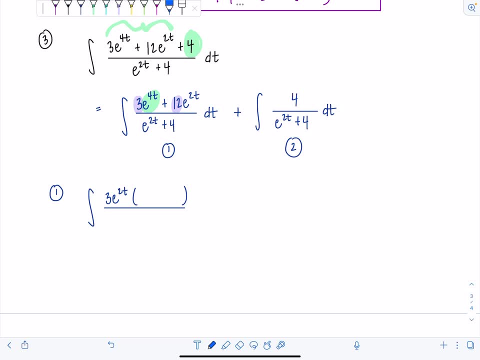 from e to the 4t. you're just going to have e to the 2t left plus plus, yes, Just a 4.. And then in the denominator we still have that e to the 2t plus 4 dt. 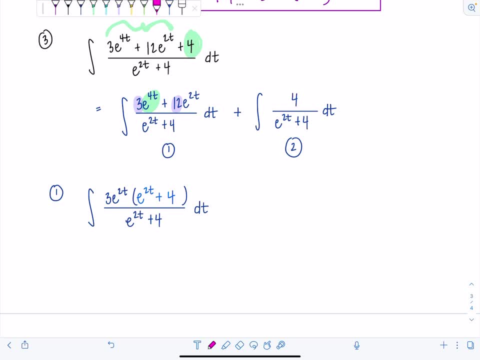 Oh, my goodness, do you notice something? I'm excited. Look at this. e to the 2t plus 4, gone, Bam, bam. And then now we're just left with integral 3e to the 2t dt. 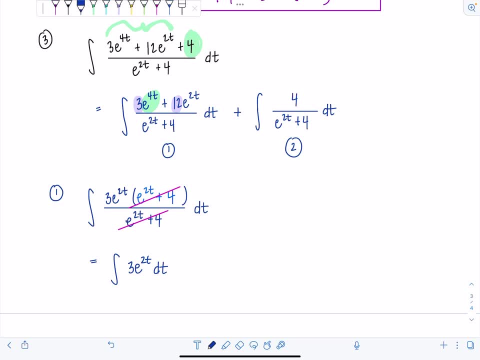 Okay, and then I hope at this point I mean, you're in advanced calculus, guys, You shouldn't need to use that. I'm just going to go ahead and do that. It's because of this silly little 2 in front of the t, right? I mean, if you waste your time, 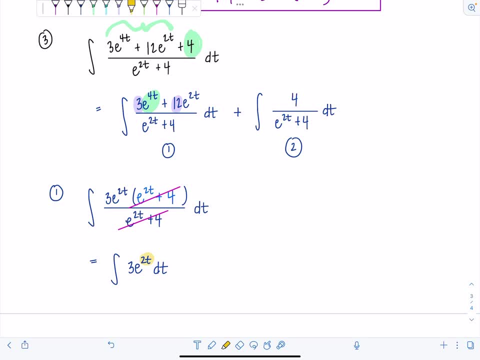 u equals 2t, du is 2dt, And then all that's going to happen is you get a one half okay. By now you should have noticed that that's what happens. So please just jump straight to the fact. this is: 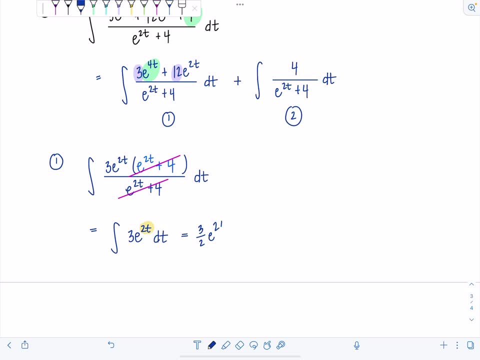 going to be three halves e to the 2t and I'm going to say plus c1,. right, I like to save that final plain old c for the final answer. Okay, Yay, integral 1 is done. That looked so painless. 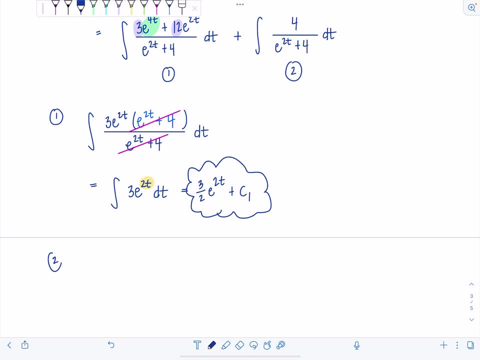 Integral 2.. What to do? So we've got 4 over e to the 2t plus 4 dt. It's not looking so cute, right? You can't just ln stuff because you see terms in the denominator. okay, Don't go down that path. That's an illegal move a lot of calc students make. 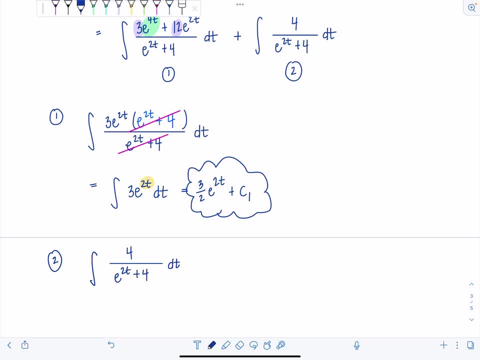 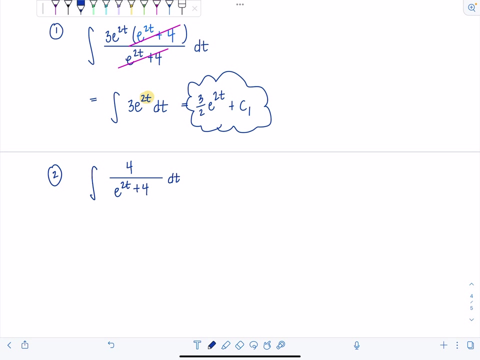 and the math police will be hot on your tail. What we're going to do is make a change of variables, use some substitution, and then we're going to end up busting out some partial fractions. Oh yeah, Here's the idea. okay, I'm going to let u equal e to the t. 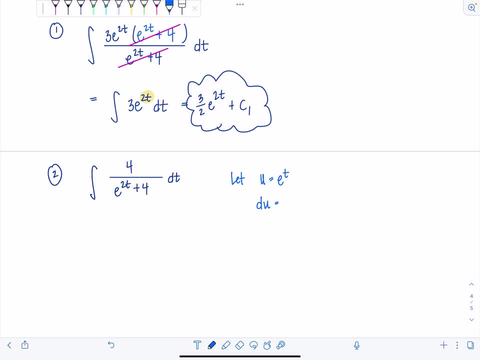 Then du would be what? Yeah, it would be e to the t dt. And you might say: I don't think that's going to work. I don't think that's going to work. I don't think that's going to work, I don't think. 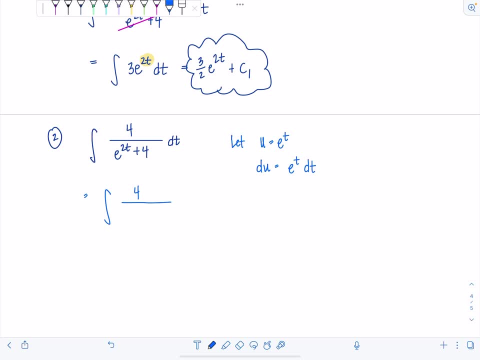 that's going to help. Well, check this out. So we've got 4 over. e to the 2t is the same as e to the t squared right Plus 4 dt. Okay, so that means we have integral 4 over if u is e to the. 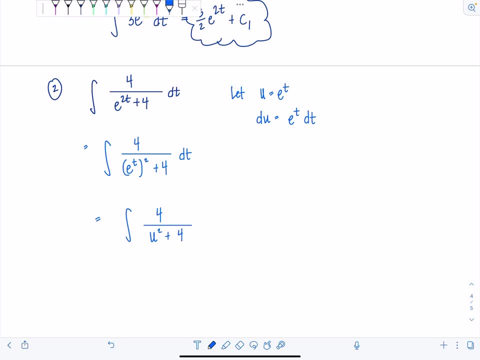 t. this is going to be u squared plus 4.. And then what about this dt? Remember So dt here is equal to du. du over e to the t. And remember: e to the t is equal to what. It's equal to u. Yes, So that means. 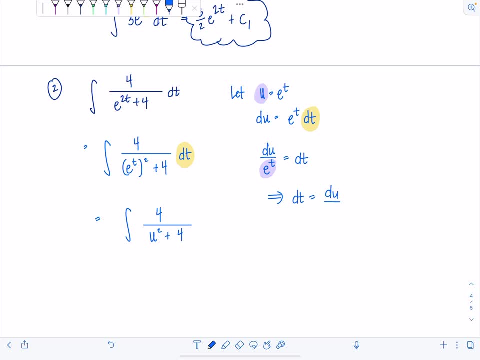 dt is equal to du over u, Uh-huh, So now I have du over u down here. Ooh, kind of weird, but I like it. Now we have integral 4 over u times u squared plus 4 du, And now we're set up where we can apply some partial 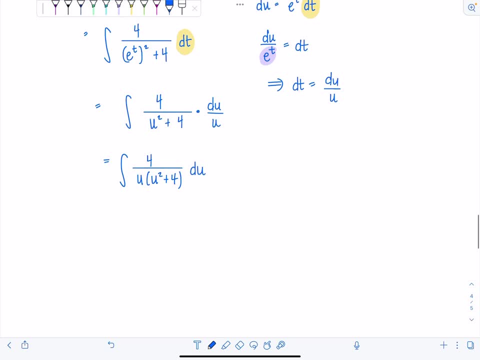 fraction decomposition, Okay. So here we go: Partial fraction time. Why don't you guys pause the video and see if you can figure out the decomposition, okay, And then check back in? All right, good, Did you pause the video? Okay? So now we're set up where we can apply some partial 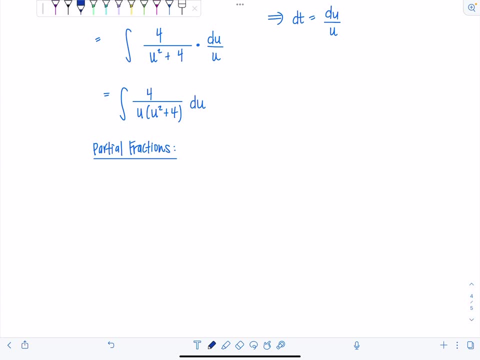 multiplication. All right, so here we go. Partial fraction time. Why don't you guys pause it? I hope you tried it yourself. It's one thing, just to sit there and watch me solve them all, It's another one. You got to do it on your own right. So we've got 4 over u times u squared plus. 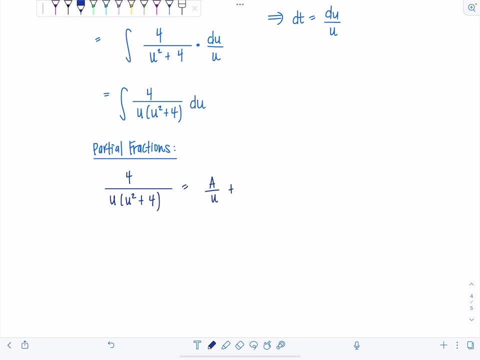 4.. That's going to equal a over u, plus you need bu plus c over u, squared plus 4, right, Good, I'm going to go through this quickly, because I'm assuming you already worked through this and you're just checking your work. So we're going to multiply by u and u squared plus 4.. And then on. 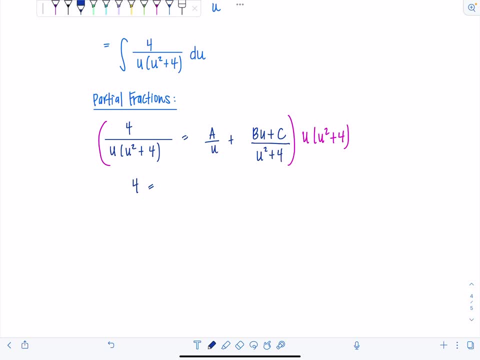 the left-hand side, we'll just have 4 equals, so the u's will cancel. I'm going to distribute right now au squared plus 4a plus, and then here this: u squared plus 4 will cancel, so I'm just going to. 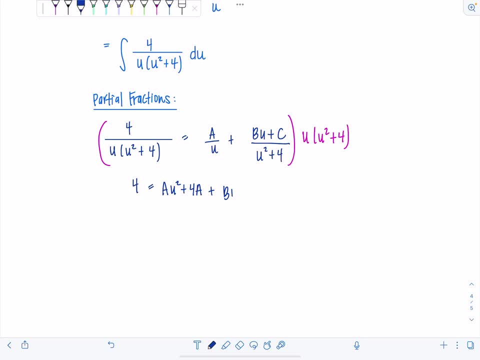 distribute the u and we'll have bu squared plus cu. Okay again, since one of the factors was an irreducible quadratic, I'm going to solve for a, b and c, like I did in the previous example, the second one. So for the squared terms, there aren't any on the left, so 0 must equal. 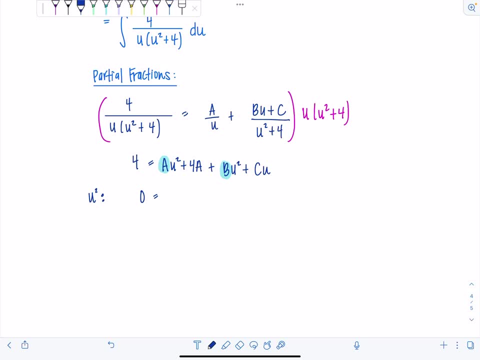 a plus b, right Good. And then the linear terms. there aren't any on the left, so that must equal c. And then constants. let's see: 4 has to equal 4, 4a. Oh my goodness, we're getting the same values as last time. How strange, or maybe not strange. 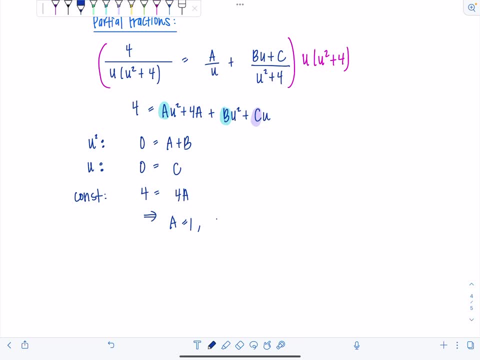 huh. So a is 1, c is 0, and b is negative 1.. Did you get the same thing? I hope so, And that means now we're left with integral 1 over u minus u over u squared plus 4. 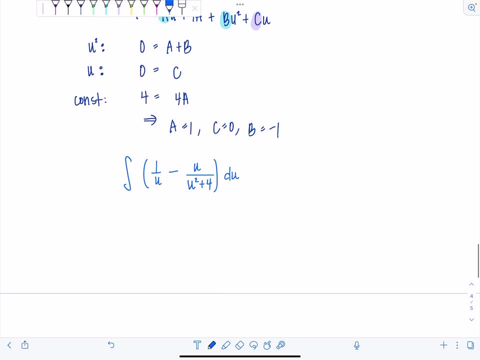 du. Okay, I'm not going to hold your hand so much. It's time to become an independent advanced calculus student. Antiderivative of 1 over u: Yes. ln absolute value of u minus. you guys, this should be super familiar. We literally just did almost the same exact. 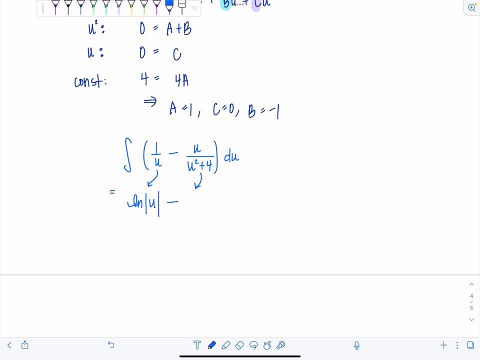 antiderivative. in the last example It's just this: 4, was a 5.. I don't want to do a u substitution. Well, first of all I can't, because I already used up the variable u, So you're going to have to pick another letter. okay, And t is used up. 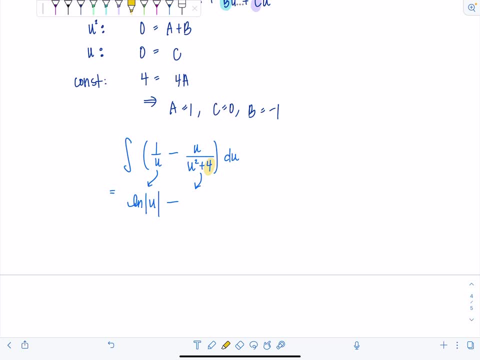 from the get-go And, honestly, at this point you should be able to recognize the pattern and not even need to do it. You're going to have a one-half ln of the denominator- and I don't need absolute value because I know this isn't going to be negative- plus c2.. 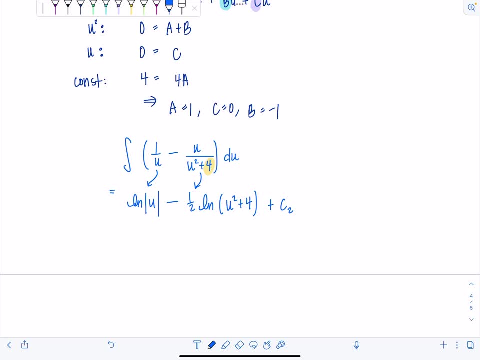 All right, If that just was whoosh way over your head. go back to the last example where I did break down the substitution so you can follow along where that one-half came from. But you should start recognizing these patterns now Because as the integrals get more complicated you don't. 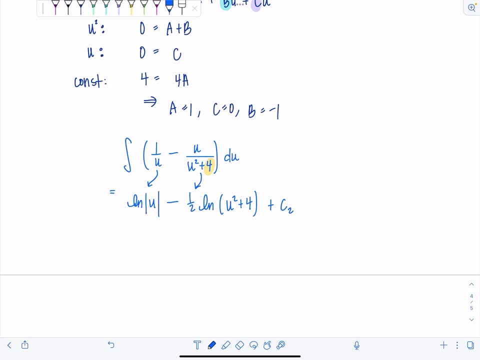 want to have to keep doing a u sub over every little baby thing. And then remember from the beginning u was equal to e to the t, So let's go back and replace that here. So ln absolute value, one-half ln of u squared- is going to be e to the 2t plus 4 plus c2.. And then ln of absolute value of 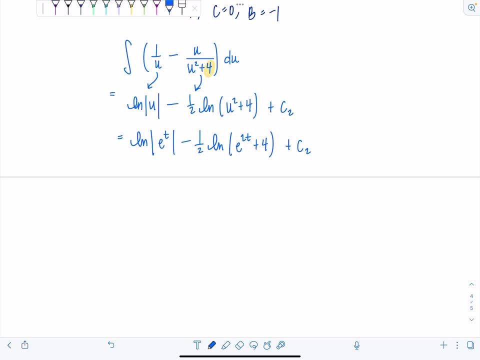 e to the t. I mean e to the t is not negative, so we didn't need absolute value there. This is just the same as ln of e to the t, which will just be t minus one-half ln. e to the 2t plus 4 plus c2.. 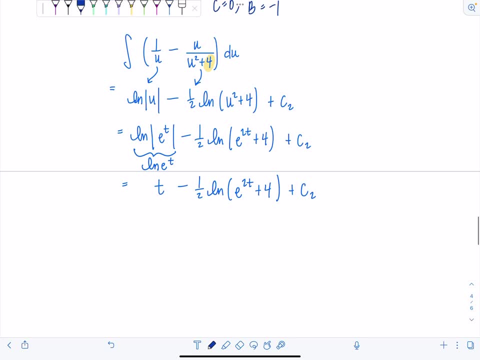 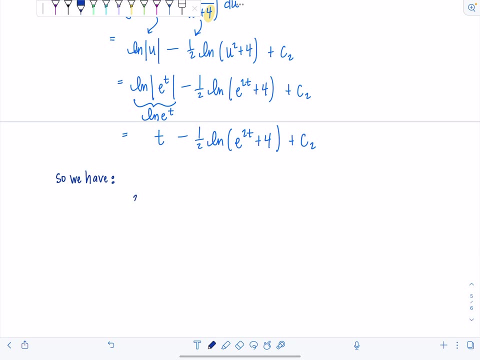 So now, final answer- because this was just the result from the second integral- is as follows: We had three-halves e to the 2t right from the first integral, plus t, minus one-half ln of e to the 2t plus 4 plus c, where c is equal to c1 plus c2.. 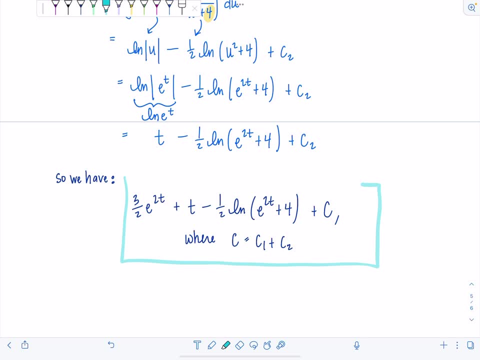 Voila, Did you like this one? It's not that bad, It's just. it looks so scary in the beginning you might think I forget it, But the plan of attack of dividing it up was really essential. Okay, so, on that note, I've got another spicy one for you, and then we'll be done. 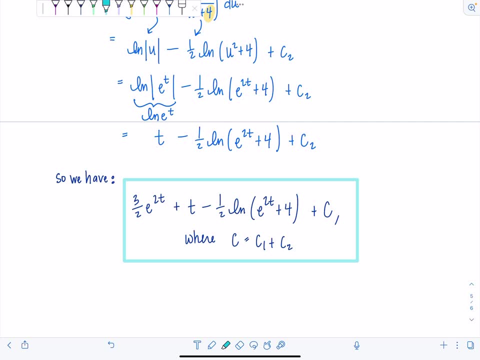 And it is kind of similar to the last one that we just did the initial approach. okay, This is like: yeah, it's Serrano level, maybe Habanero, I don't know. We'll have to find an appropriate pepper to classify it. You can let me know in the comments. 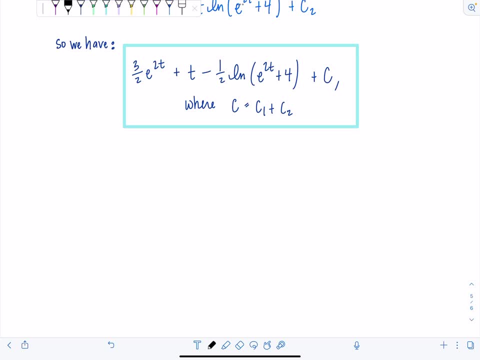 your rankings of them. okay, and the appropriate chilies. Example four: It's going to look frightening, Please don't be scared. We've got integral Integral. I love these. Okay, x plus 5 squared tan. inverse of t. 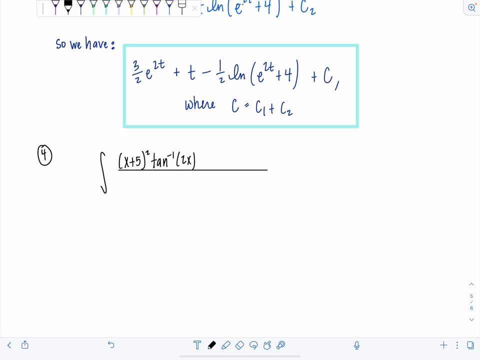 Inverse of 2x plus 4x cubed, plus x over 4x squared, plus 1 times x plus 5 squared dx. Holy moly. Okay, I already gave you a hint that you're going to break it up. 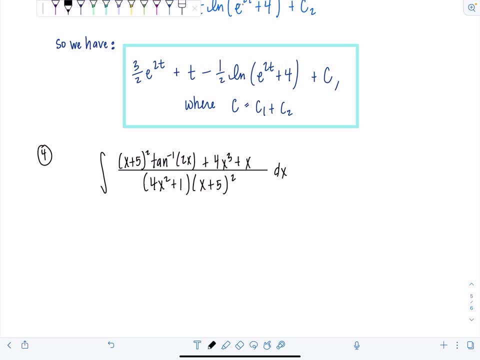 You know how do you want to group things this time? You see how this has an x plus 5 squared in it, as does this denominator. Let's split it right here. You see what I'm saying. I hope so. Here we go. 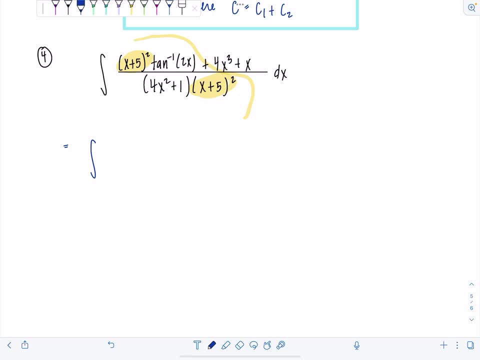 Two integrals We've got. first one x plus 5 squared tan. inverse of 2x over 4x squared plus 1,. x plus 5 squared dx. x plus 5 squared. x plus 5 squared dx. 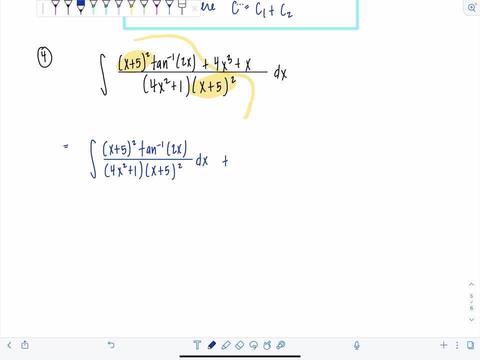 x plus 5 squared x plus 5 squared dx. x plus 5 squared x plus 5 squared x plus 5 squared dx- squared dx plus. that's the first integral. second integral is going to have 4x cubed plus x in the 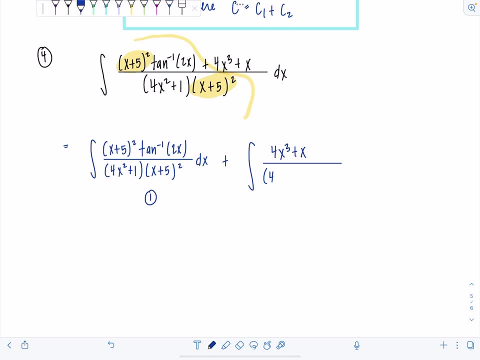 numerator over 4x squared plus 1, times x plus 5 squared dx. Okay, let's tackle them one at a time. Are you ready? All right? first one: Anything you notice with integral 1?? Remember we split it up a. 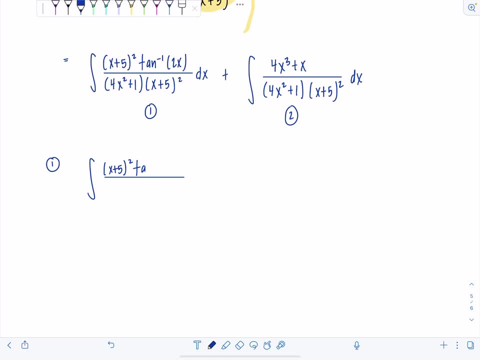 certain way because we wanted to cancel some stuff out. right Yeah, so the x plus 5 squared will cancel out. So let's go ahead and do that. Bam bam gone, And then things should start looking kind of interesting. 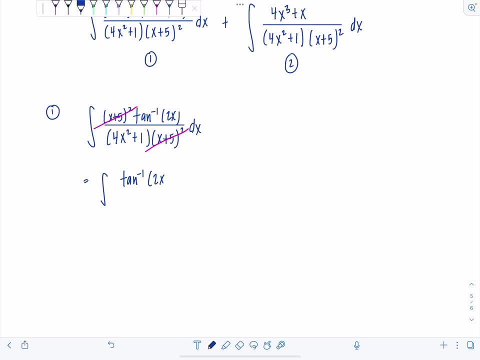 Somewhat familiar. I mean, we've got a tan inverse of 2x, All right, And then this 4x squared plus 1 in the denominator, And I'm feeling a use of. Why am I feeling that? Because I know. 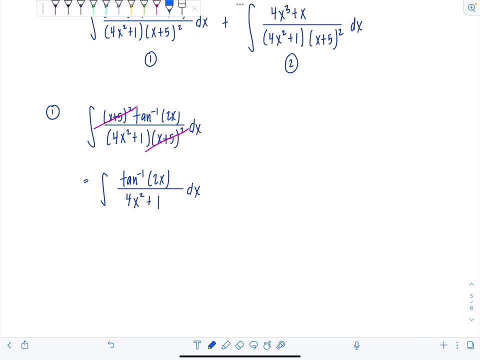 I learned my derivatives a long time ago and I made sure I memorized them. The derivative with respect to x of tan inverse of x is 1 over 1 plus x squared, And so, since I have a 2x here, that would mean this would end up being a 4x squared, which is exactly what I see in the 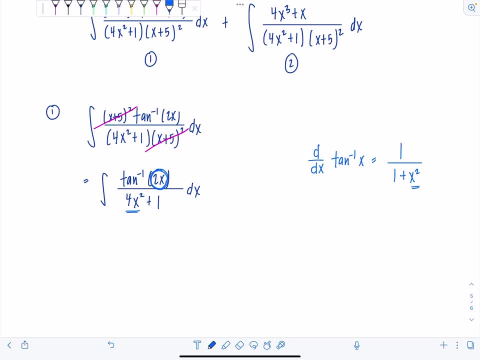 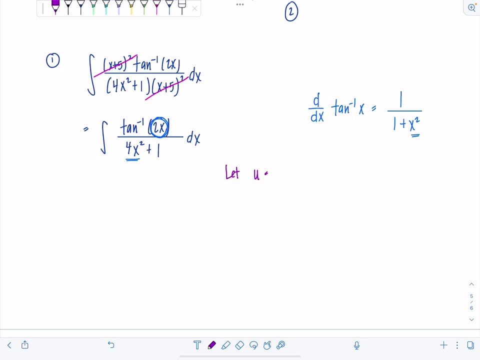 denominator. So I feel like u sub will work out beautifully with this problem. In that case, we're going to just let u be the denominator, the numerator, excuse me. So let u equal tan inverse of 2x. And then just be careful when you find du, because we have to use the chain rule, right? 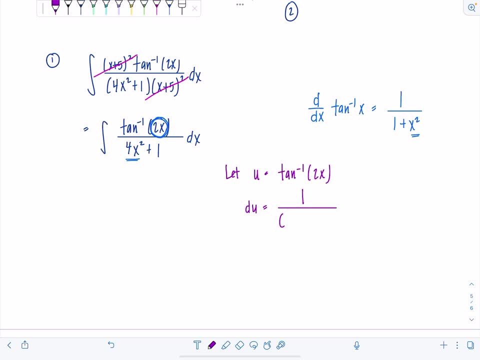 So you're going to have 1 over 2x squared plus 1 times. What's the derivative of 2x? It's 2.. So don't forget that dx. That's not exactly what we have. I'm going to have to move. 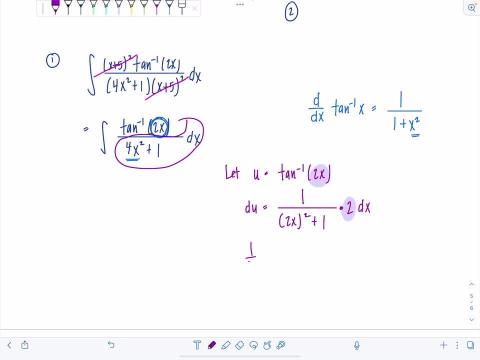 this 2 over to the other side. So 1 half du is equal to dx over 4x squared plus 1.. Oh, do you see it now? Ooh, okay, So here we go. We've got that 1 half. Let's put it outside integral in the numerator. 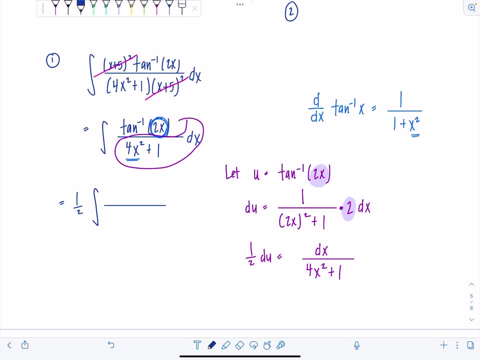 instead of tan inverse of 2x. just sweet little u minding its own business. You know what? I don't even need a fraction bar, huh. And then that kidney bean that I drew right here. that was my 1 half du. I already got the 1 half outside du Bam. Wow, wow, wow. This is such a nice little. 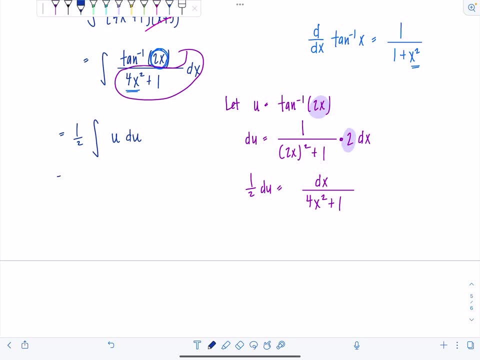 integral Anti-derivative of u: 1 half u squared. We already have a 1 half sitting outside, So this is 1 fourth u squared, plus that's right, c1.. And then just go back. We're going to replace u. 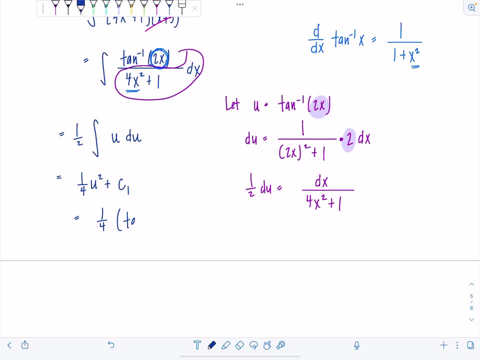 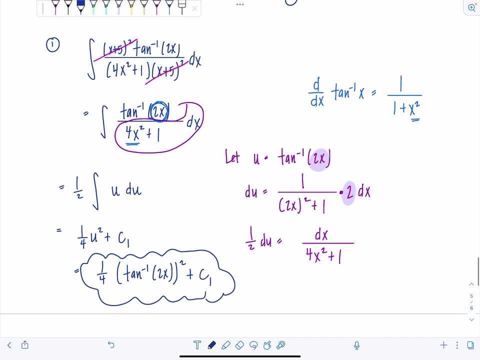 with what it originally was. What was it Tan? inverse of 2x squared plus c1.. Okay, Integral 1 is done. Nice, Now let's move our attention to integral 2.. You see it: 4x cubed plus x over 4x squared plus 1. 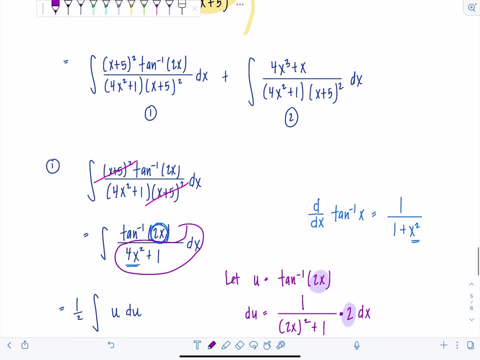 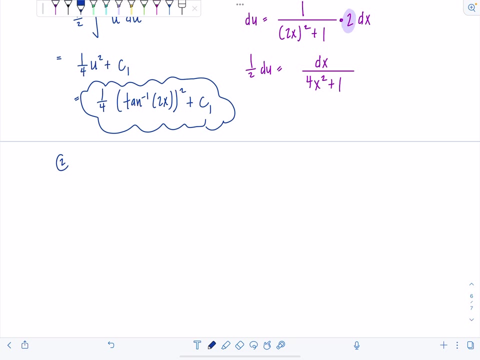 times x plus 5 squared. I want you to notice. you could take an x out here. Did you see that? initially? Maybe not. Maybe you were so traumatized, huh, Okay, So let me rewrite it now with the numerator factored so you can see. So we've got integral x times 4x squared. 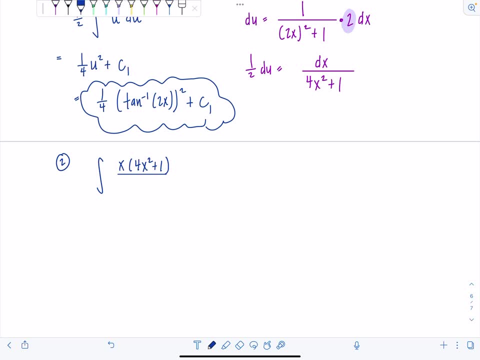 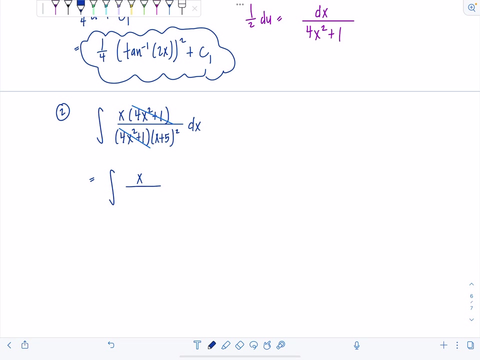 plus 1 over 4x squared plus 1 times x plus 5 squared dx. Yay, Look what we can do, you guys. Cancel out this 4x squared plus 1.. Fabulous, Okay. Then we have integral x over x plus 5. 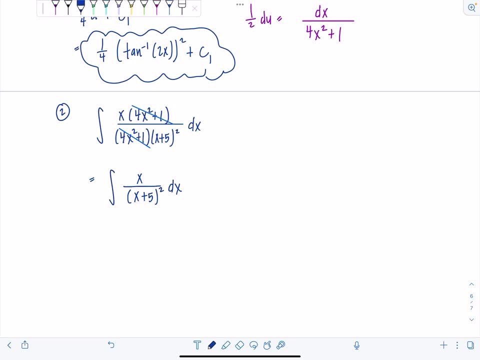 squared dx. Okay, Now from here you've got some options. Yeah, You can do partial fraction decomposition for x over x plus 5 squared. Okay, If you did notice, in the denominator we have a repeated linear factor, So the setup would be as follows: x over x plus 5 squared equals a. 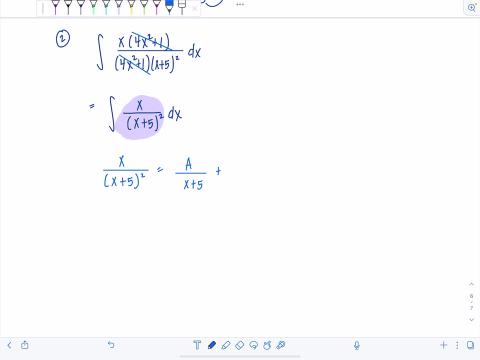 over x plus 5 squared. Okay, So we have a repeated linear factor. So we have a repeated linear factor. We have a repeated linear factor. So we have a repeated linear factor. So we have a repeated linear: 5 plus b over x plus 5 squared. okay, So that's one way you could do it. Then you would multiply. 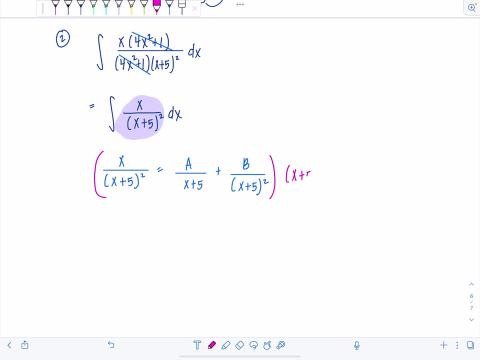 everything by x plus 5 squared and be done. I'm going to show you something else, just so you have more tricks up your sleeve, okay, Or you could do this: We have x over x plus 5 squared, and what I'm going to do is add 5 and subtract 5 to the numerator And then watch how I'm going to regroup. 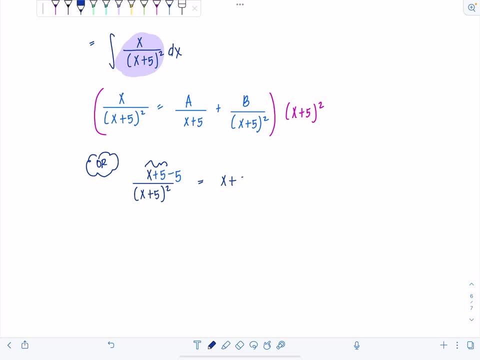 the terms. So I'm going to put this x plus 5 over the denominator x plus 5 squared and then I have minus the other 5 over x plus 5 squared And the whole point of doing that is now the x plus 5 in. 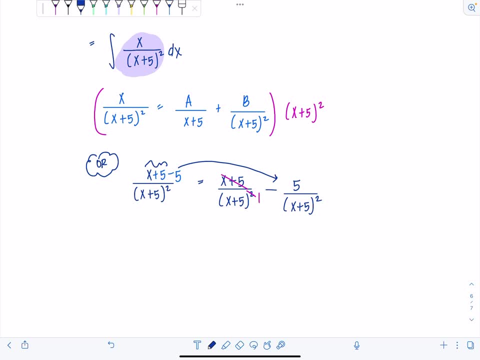 the numerator will cancel with one of the ones that are on the denominator. So I'm going to one's in the denominator. So we have 1 over x plus 5, just to the first now, minus 5 over x plus 5 squared, And that's what you would get if you sat there and did the partial fraction. 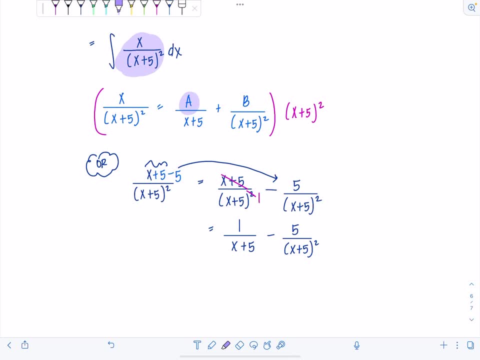 decomposition, A would be 1 and B would be negative 5, okay. Sometimes doing this plus or minus 5 business, though, makes students nervous, So you don't have to do it. I just want to show you some options. It's pretty slick, though, right? I always feel a little fancy when I bust out that maneuver. 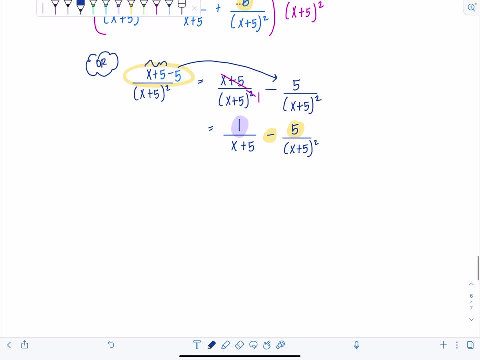 Okay, so from here, if you hated that, then just do the partial fractions, Make sure you can get the right combination, And we're going to be integrating 1 over x plus 5 minus. you know how I'm going to write the next. 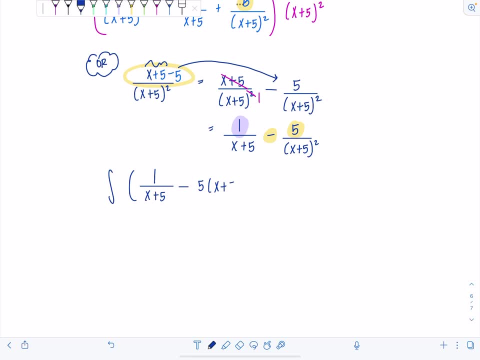 term for you. I'm going to write it as 5 times x plus 5 to the negative second dx. Okay, Anti-derivative of 1 over x plus 5?. Mm-hmm. ln. absolute value x plus 5.. And you guys? 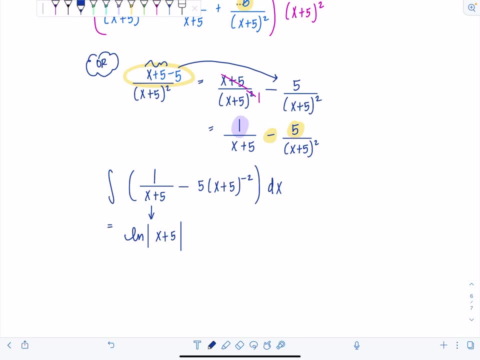 please do Not you sub for this next one. You should be able to anti-differentiate this in your head: x plus 5. If you were just integrating x to the negative second dx, you would add 1 to the exponent divide by the new exponent, which is the same as just multiplying by a negative 1,. 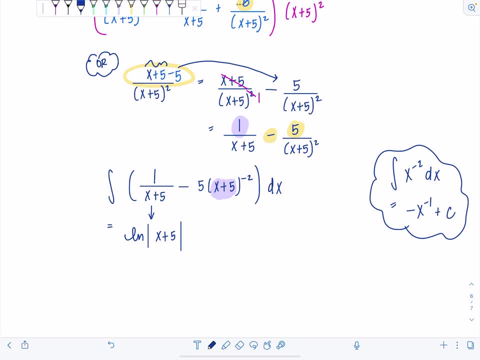 right And you'd have plus c. Well, does it make a difference that now we have x plus 5 instead of plain old x? If you sat there and did a sad little, you sub. I say sad because I mean it's really just a waste of time. If u is x plus 5, du is dx. 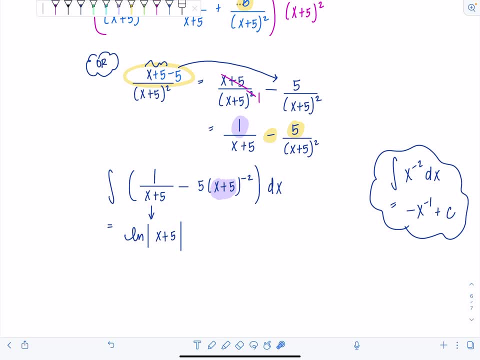 all that you're accounting for is this plus 5.. I mean, who cares? Can't we just account for that as is? So now we're going to have plus 5 times x, plus 5 to the negative first. Yeah, Do you see it? 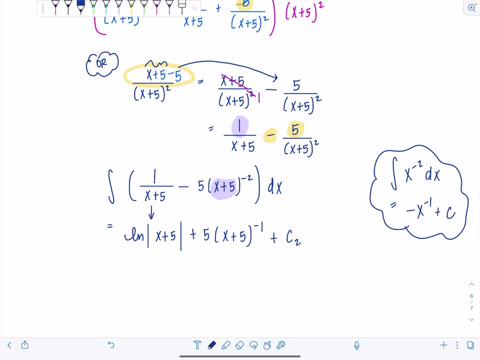 I hope so, Plus c2.. And of course I'm not going to leave it like that. It looks so gross. So ln: absolute value x plus 5.. I'm going to add a negative first. I'm going to add a negative first. 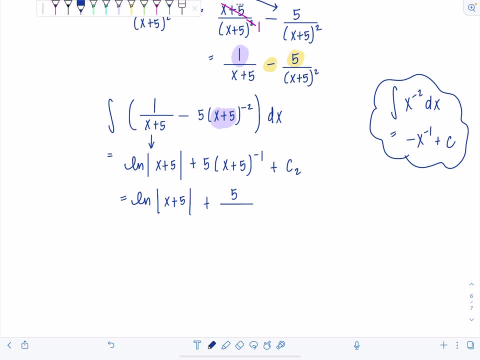 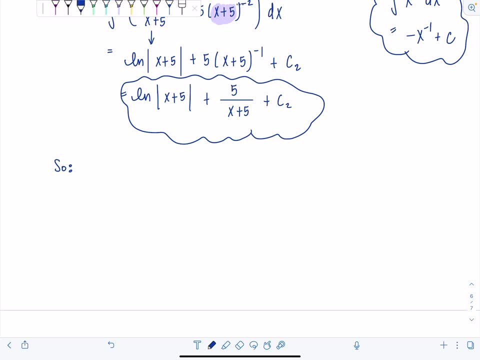 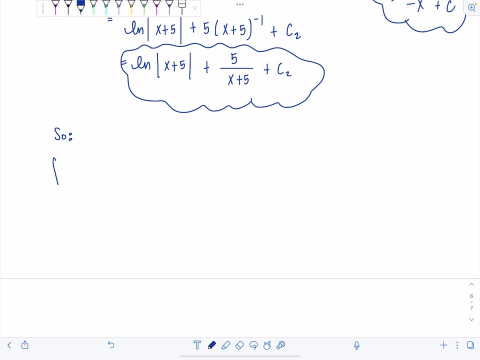 it all together. I feel like we forgot what the original integral was. did you forget? let's rewrite it. just to be such thorough, little mathematicians: integral, what was it? it was scary. x plus 5, squared tan, inverse of 2x plus 4x, cubed plus x.